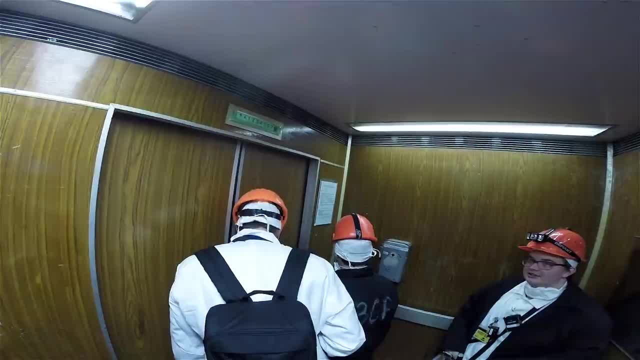 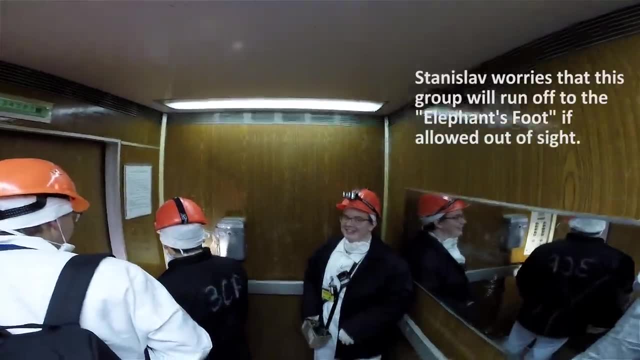 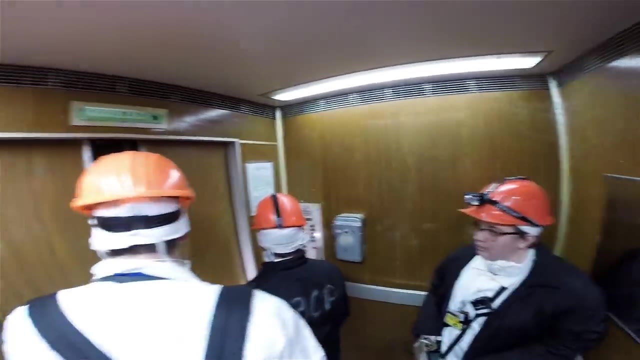 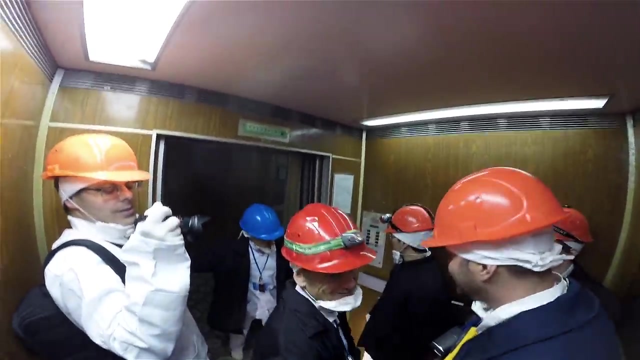 Yes, Yes, Stassi. Okay, what button is for the phone? What? So? here is level 9.2.. Push button: 9.2.. Alright, Yes, Hello, Maybe we go upstairs by walk, because I am not sure that we will go there. but 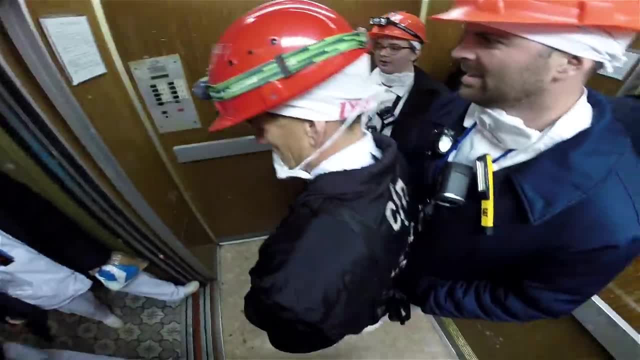 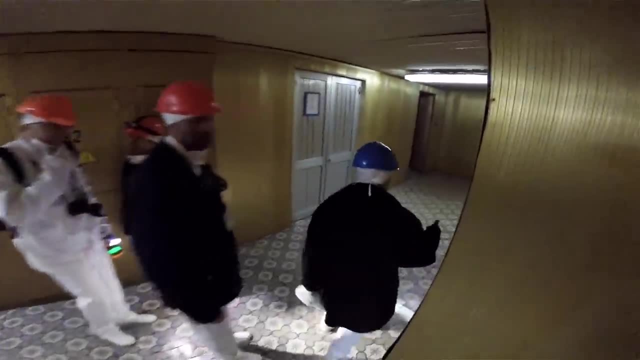 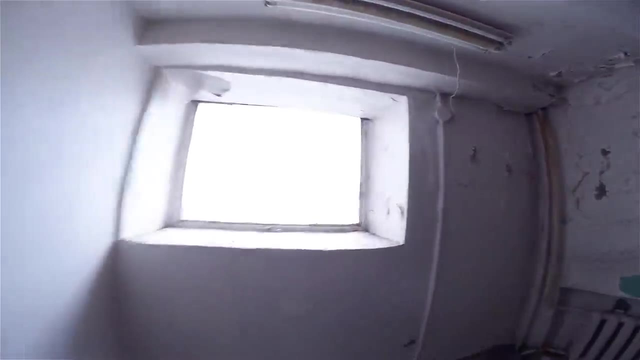 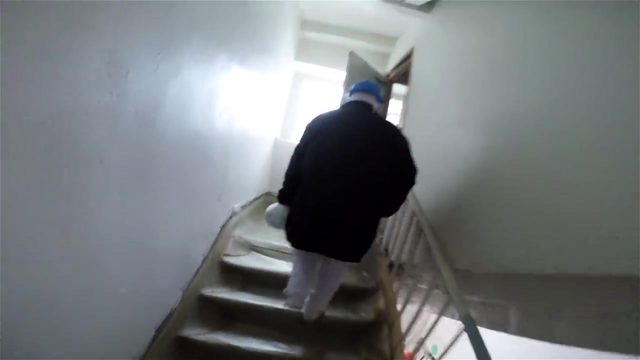 Yes, Okay, Go, go, go, go, go, go go, Because we She has some problem with it. Let's go upstairs, Let's take the stairs. I am afraid that the elevator It is possessed. Yes. 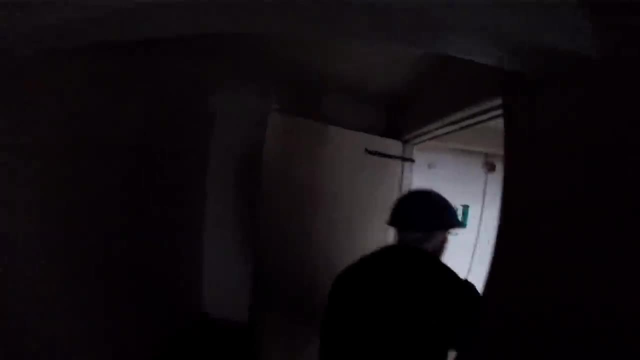 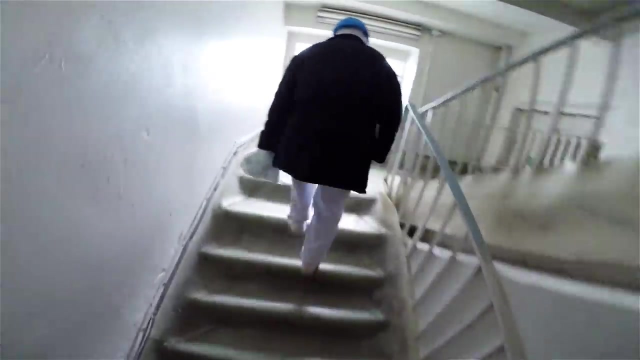 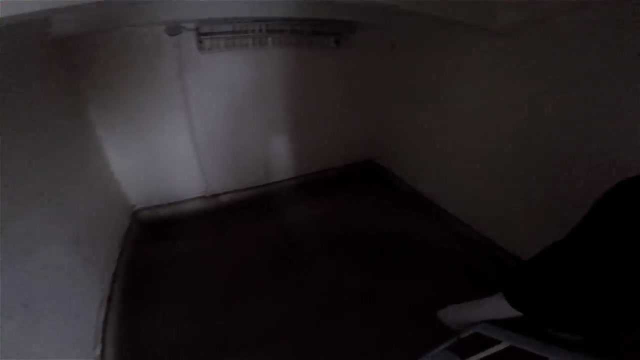 So we'll work our way up this stairwell to the 20 meter elevation and get off there to go visit the central hall. Um, We need metal. This is our escort here, Stanislav Shekstilo, a long-term employee here in the information department at JNPP. 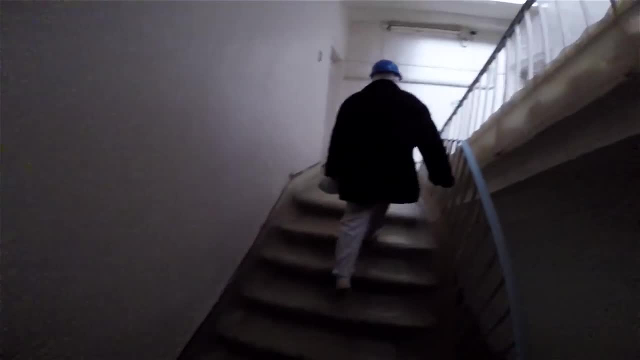 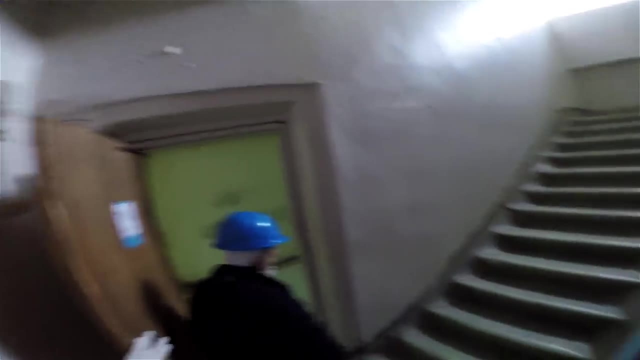 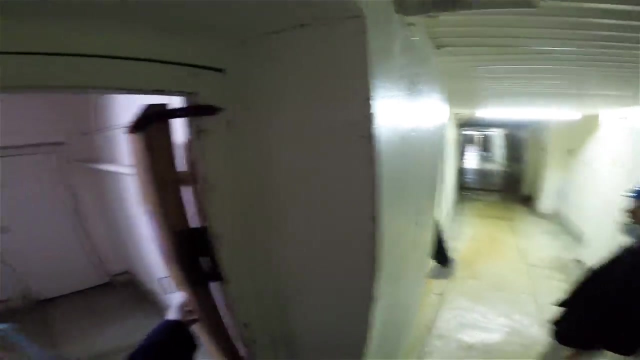 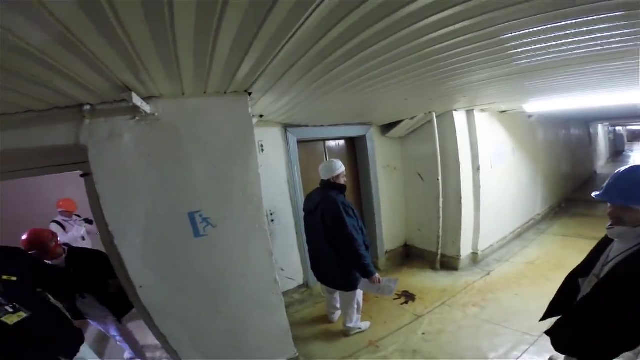 He has been here since the days that this was an operational nuclear power plant. He has been very good to us. We We Frustrate him sometimes, I think, asking to do things like: oh, visit the elephant's foot, and things like that. 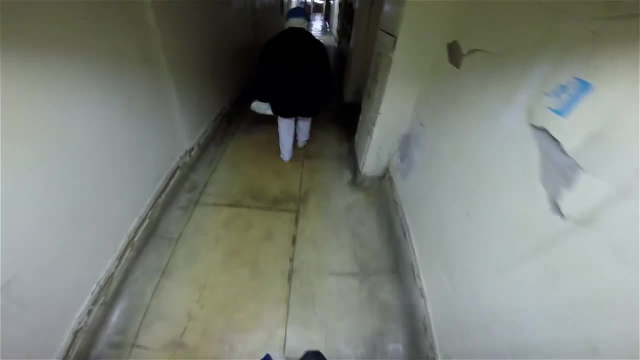 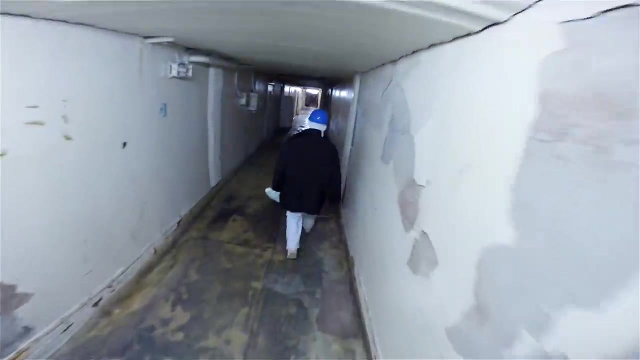 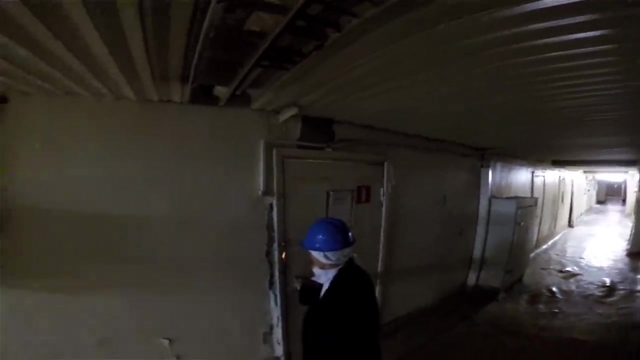 He is, He plays right along On the left. here are going to be the compartments for the drum separators in this type of reactor, And then we'll come here to the enter room, to the central hall where people change clothes and so forth, to work in the. 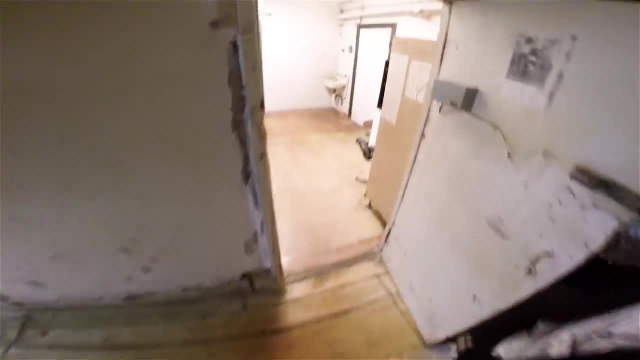 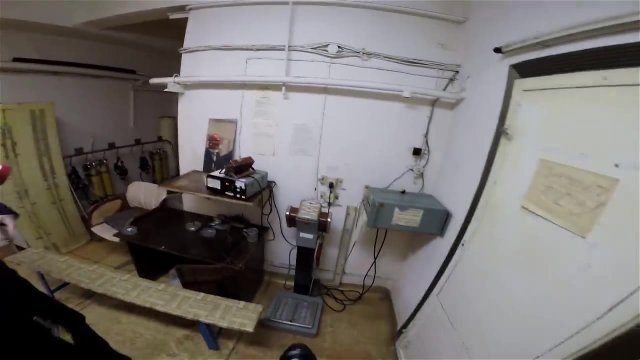 At the reactor fueling phase. Um, So we'll come on in here. There's some radiation detection gear, because the central hall is a fuel handling area and is potentially radioactive. Um, There's a bench for changing boots and gloves and so forth. 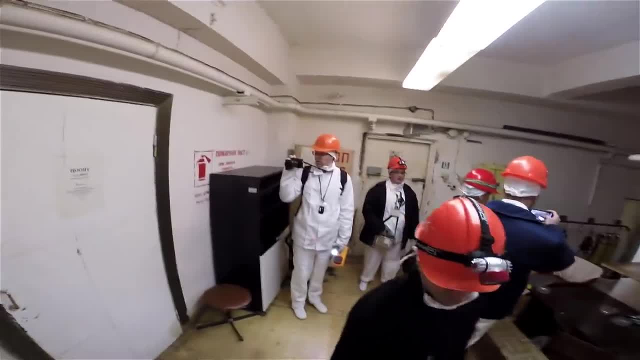 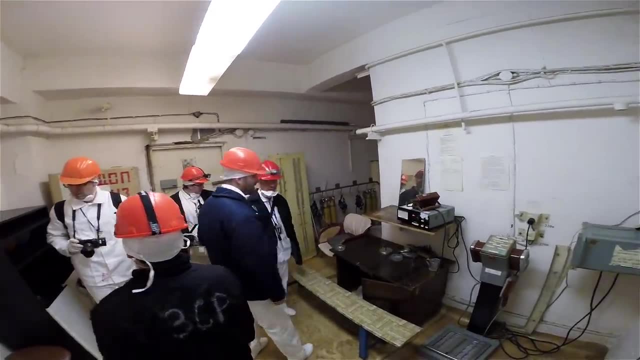 I'm not going to show you the whole process, because it's pretty boring watching people put on boots and gloves, But we'll speed up here and then look at some other stuff. once we go in, Uh-huh, I'll get pictures, Shh. 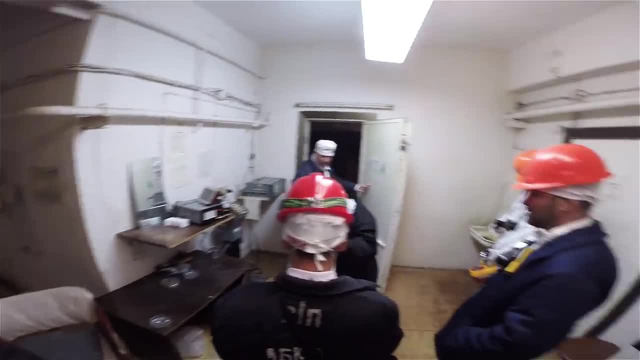 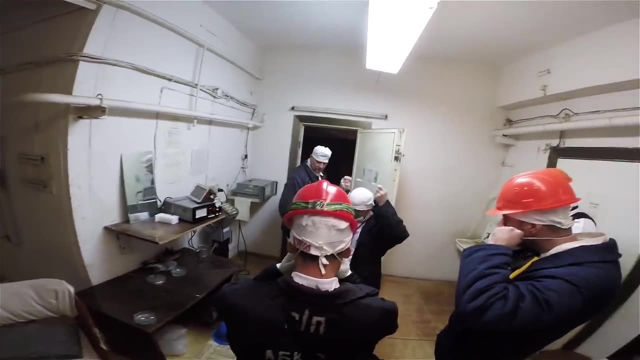 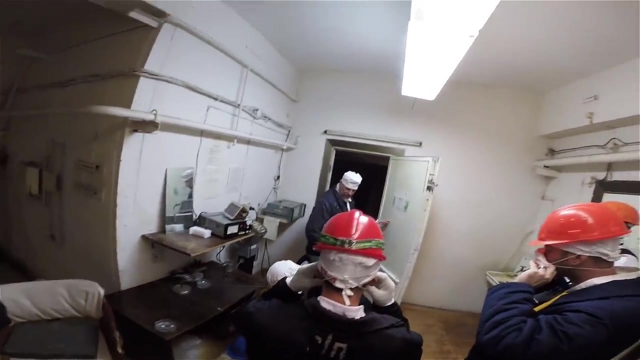 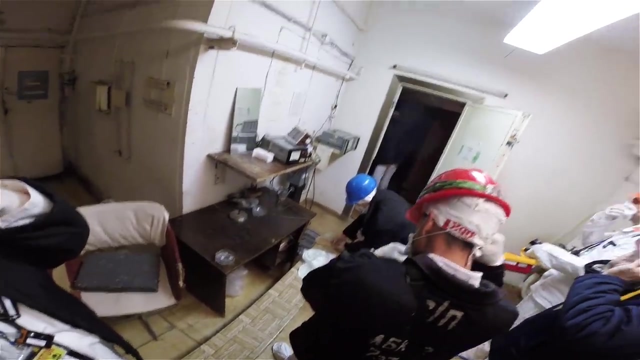 Uh-huh, Uh-huh So, and also respirator, Naturally. So be attentive please during our So being here in the reactor hall. be very attentive please, Usually as usually. Yeah, Yes. 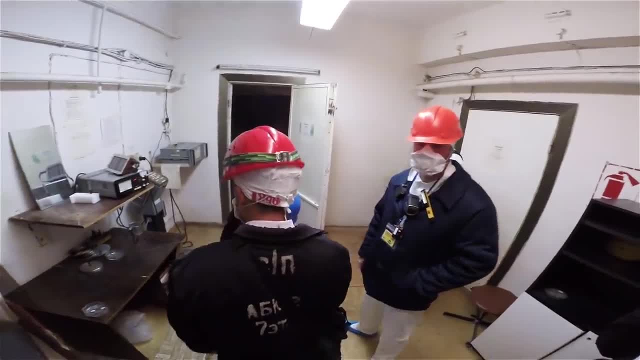 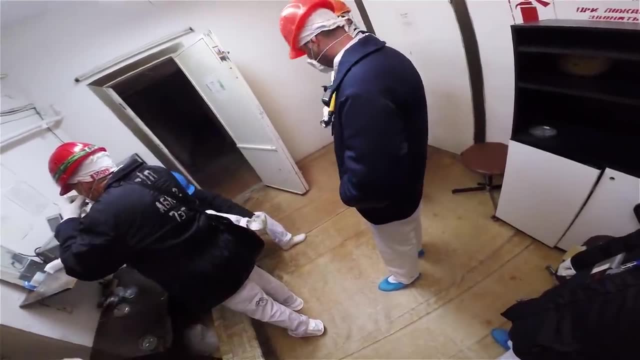 Uh-huh, Okay, So that's my. It might be backwards, Uh-huh, Oh, it is. That's yeah, Yeah, the little padlock in the back. It's okay. It's okay, I know. 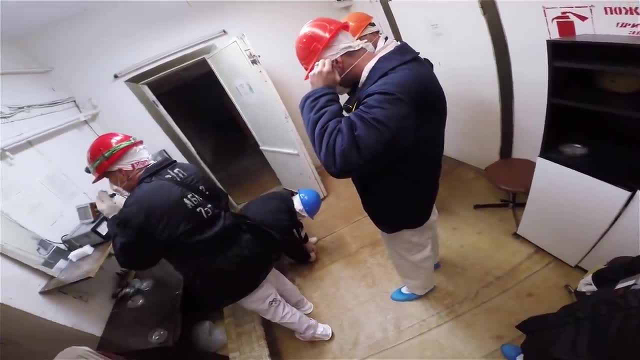 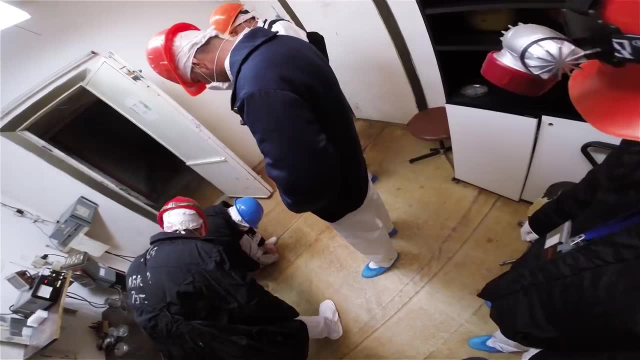 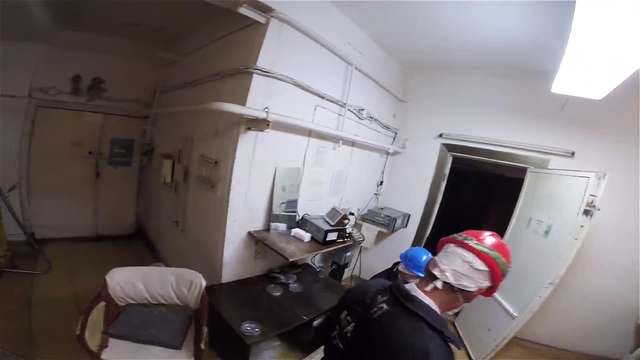 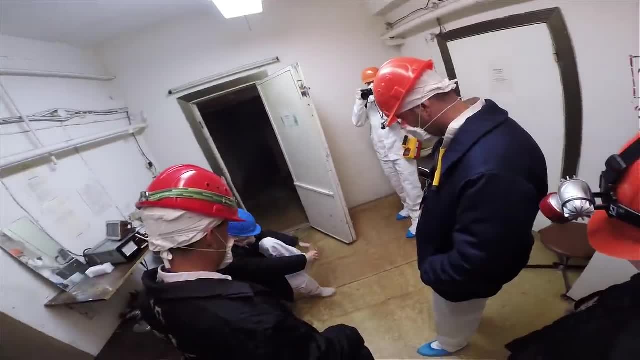 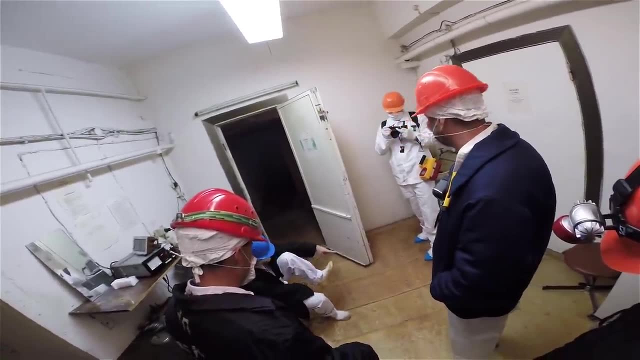 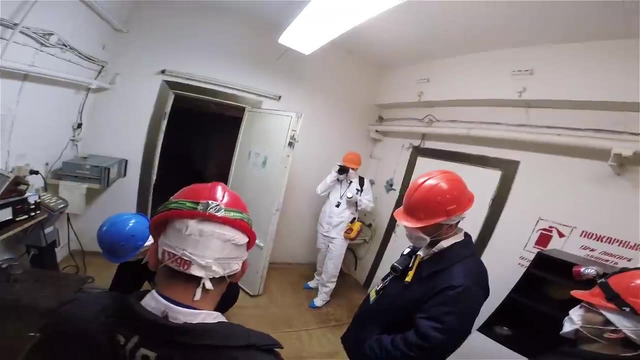 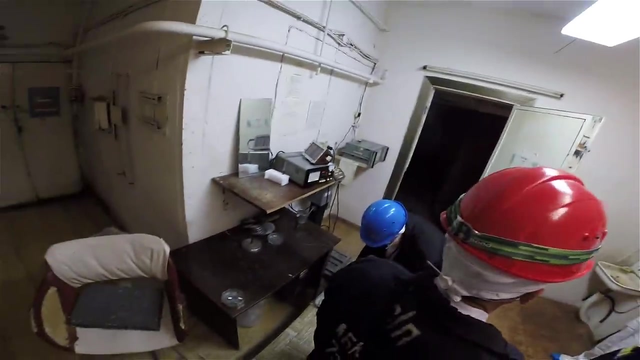 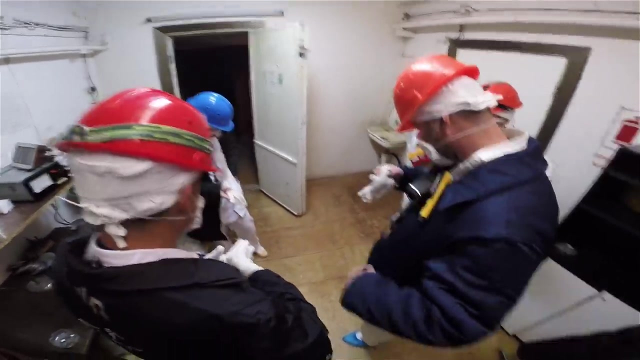 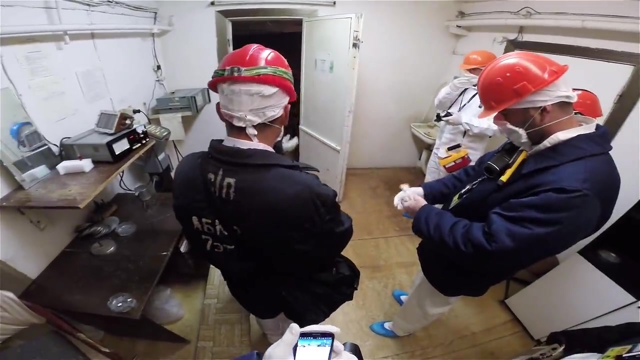 It's better to do it like this, because they are too big, It's not 45 or 43,. you see, Yeah, as long as you have it Ready, Ready, So we're heading in. The Central Holocaust is not only a contamination area. 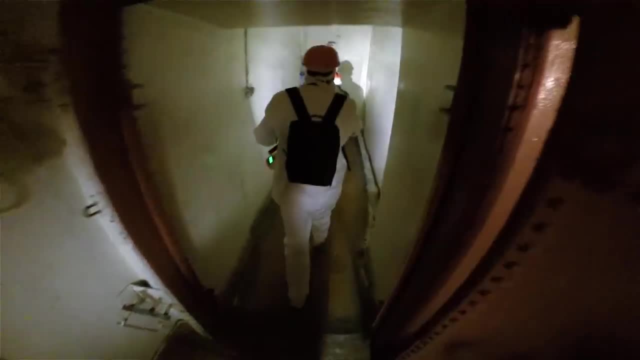 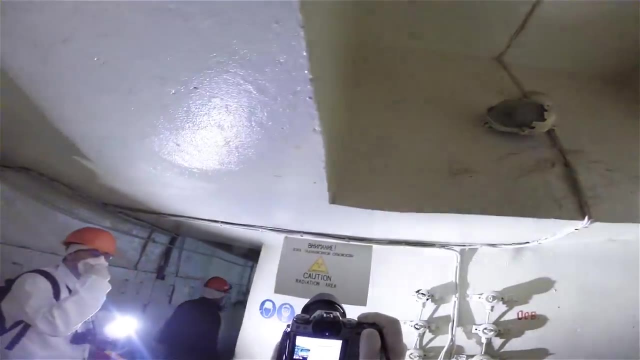 but also a giant hot cell for fuel handling, because when the fuel's out it produces a lot of radiation in this area. So, you'll note, we go through this little dogleg of concrete that acts as radiation shielding and then we'll step into the. 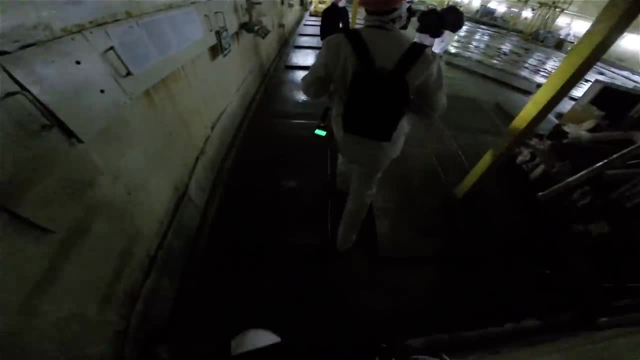 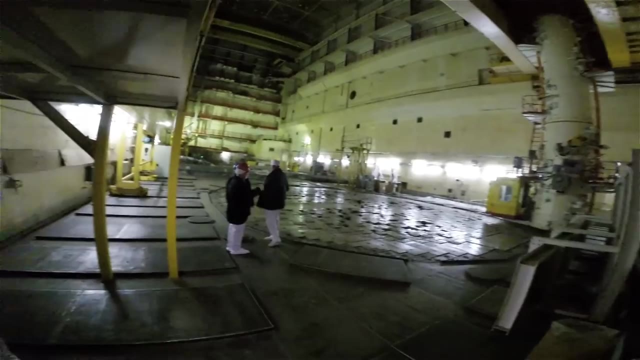 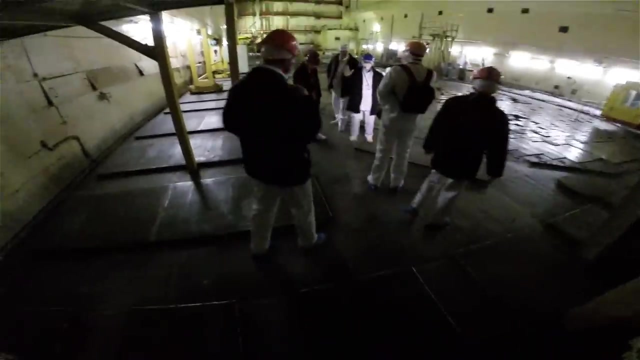 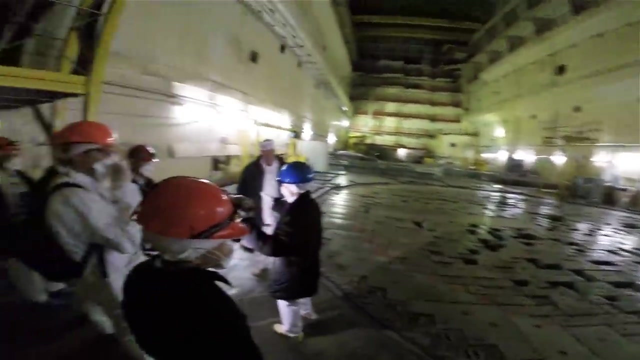 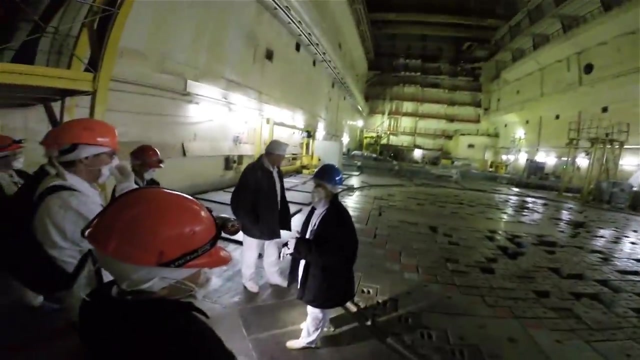 central hall itself. And here we are. So this is a small information again for your attention here, my own work, because something is open, and the request of this operator not to go here on the upper corner of the reactor. 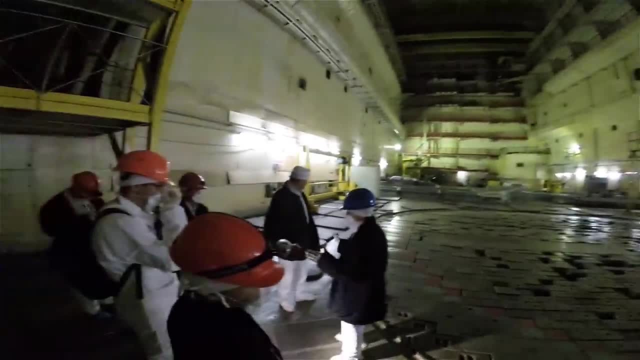 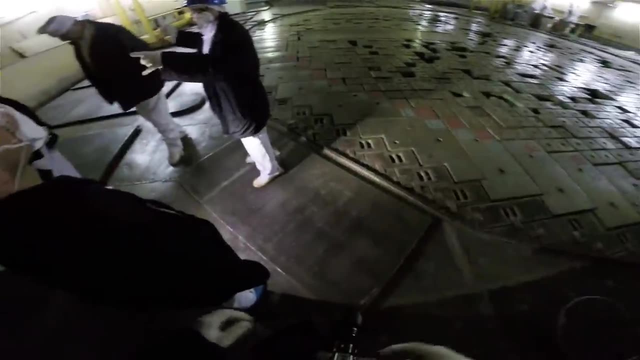 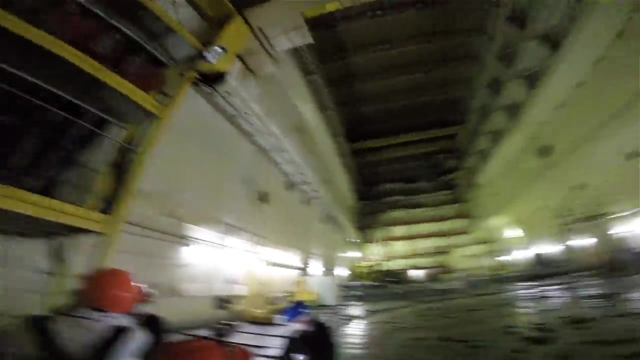 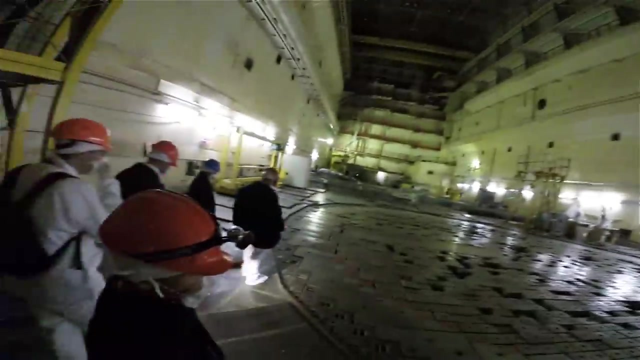 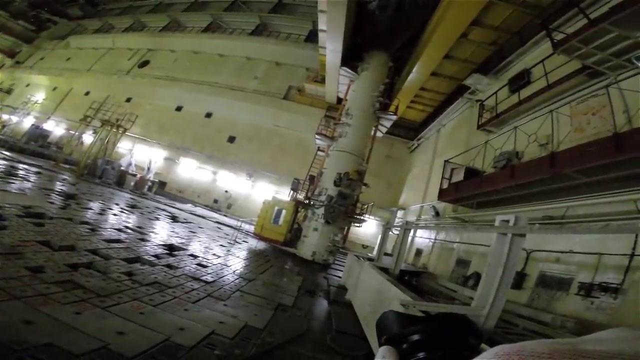 You can go round round and also like this, And I'll ask him to switch off the light. Oh, thank you, Thank you. Look at that fuel handling machine Like a rock. The RBMK reactor is constructed from graphite blocks. 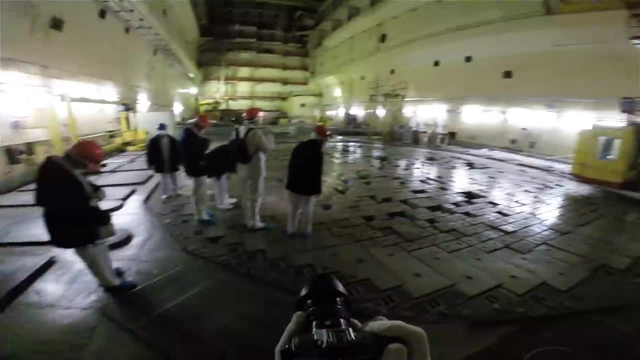 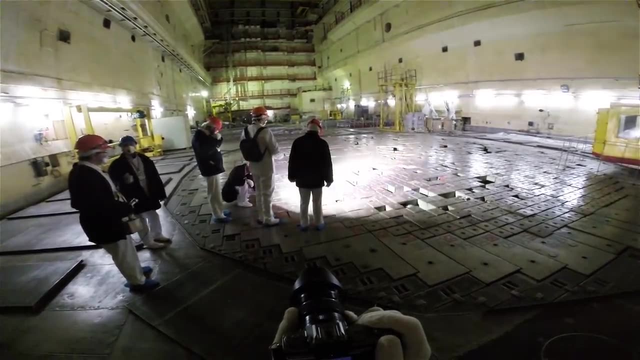 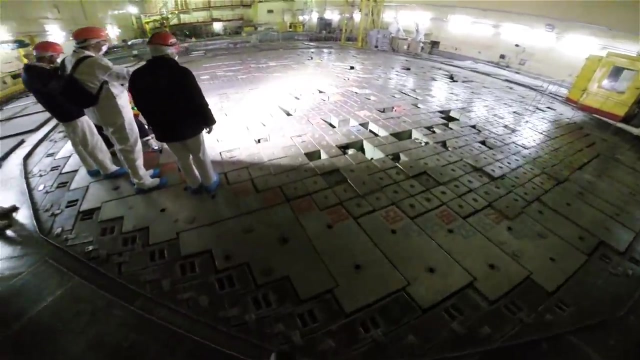 that are penetrated vertically by pressurized tubes that carry the nuclear fuel and other in-core devices like control rods. And what we're looking at here is the top plate of the reactor, where it's been penetrated by all of these channels And there is a protective 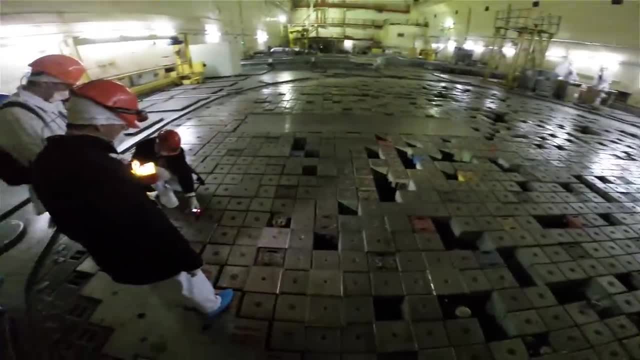 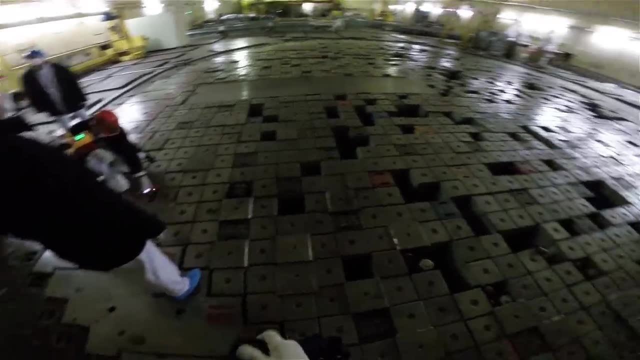 heavy metal cap over each of the channel penetrations to protect it from mechanical damage. The reactor is empty right now. There's no fuel, It's all been taken out, And there's also no water, So actually there is a little bit of radiation up here. 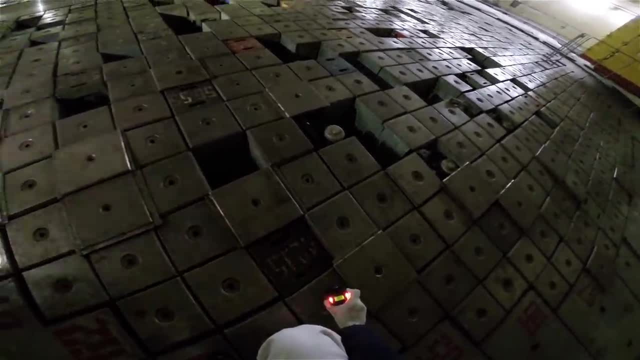 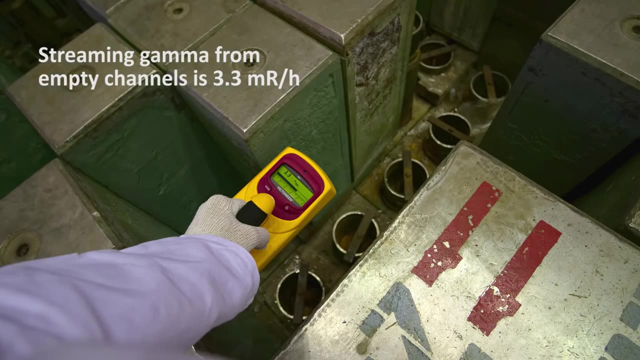 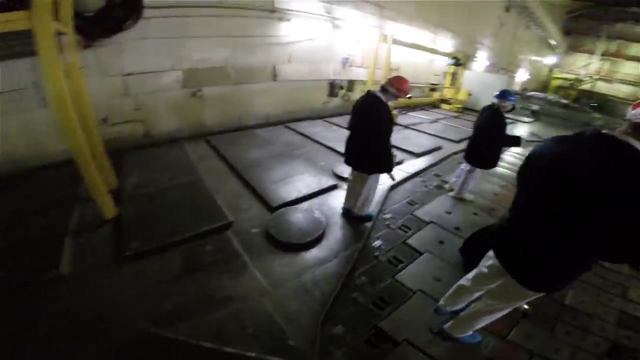 And it's due to radioactive material down in the channels And the radiation is streaming up through the empty channels and up to the fueling face. where we are now Over here on the side are a bunch of heavy steel plates that cover up the steam water pipelines. 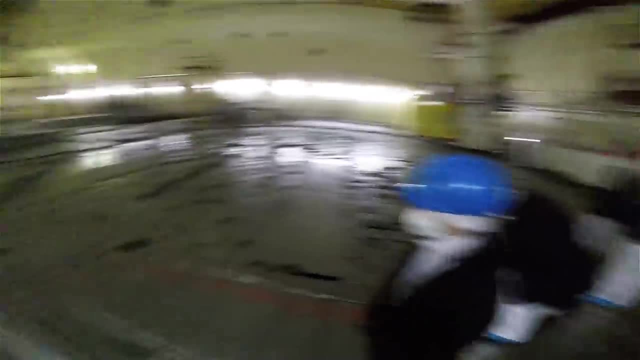 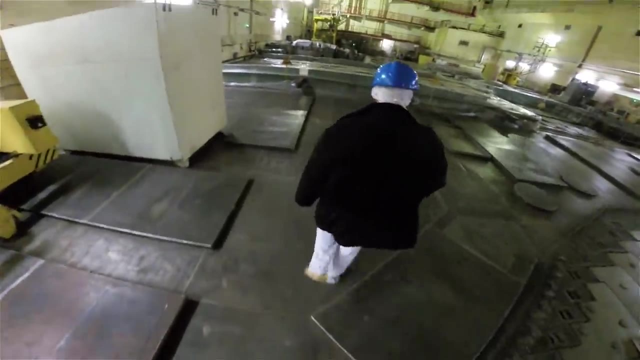 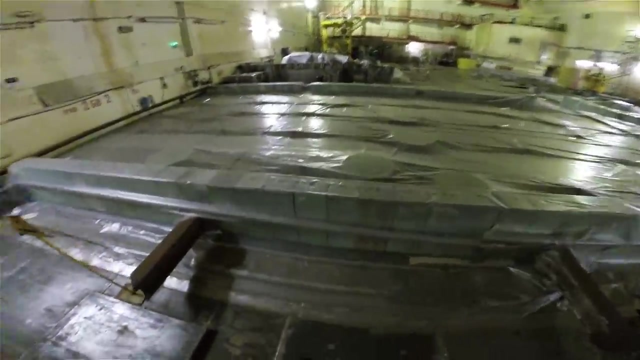 from the upper part of the reactor And they will go under the wall on either side of the central hall and bring steam to the drum separators. Over here are some caps for the technological channels. They're a little bit radioactive just because of their proximity. 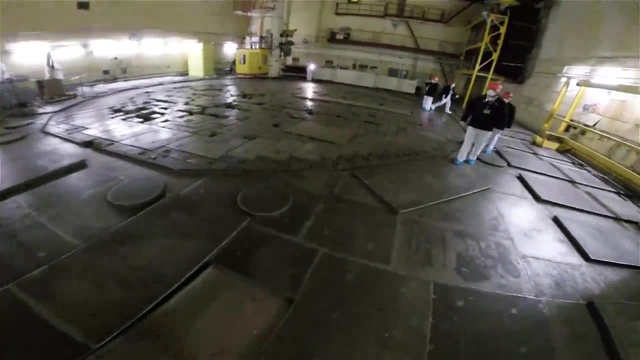 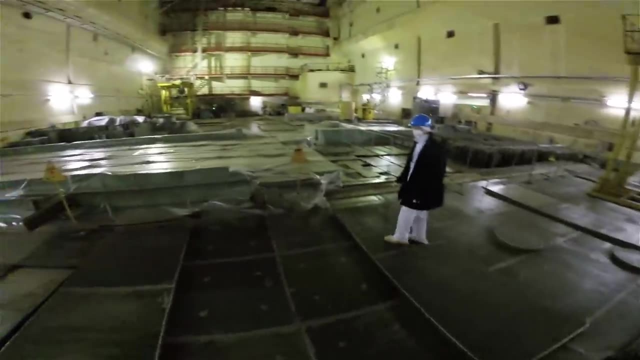 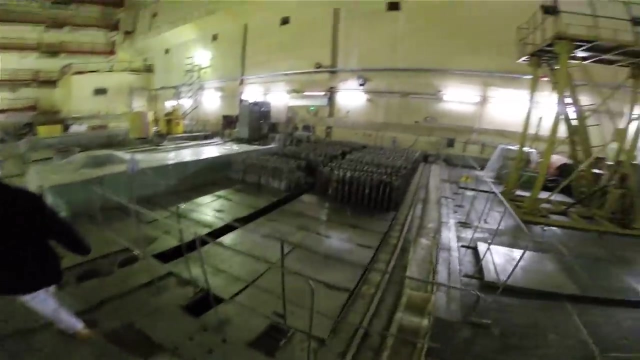 to. you know dirty stuff, But they again provide mechanical cover to the channels up here on the core face. We're going to go ahead and pass between the two spent fuel pools. There is no fuel in these pools. It's all been taken out to ISEF-1.. 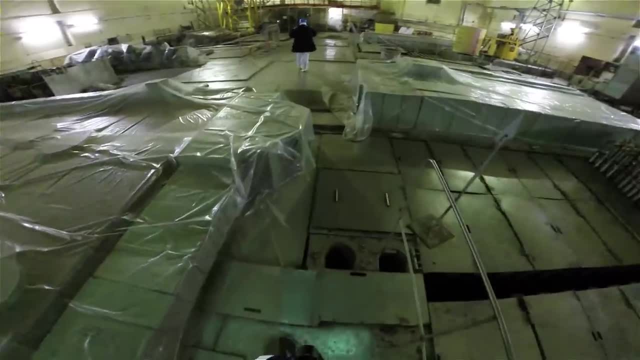 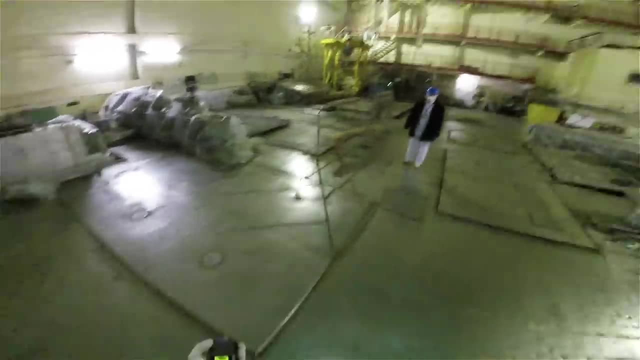 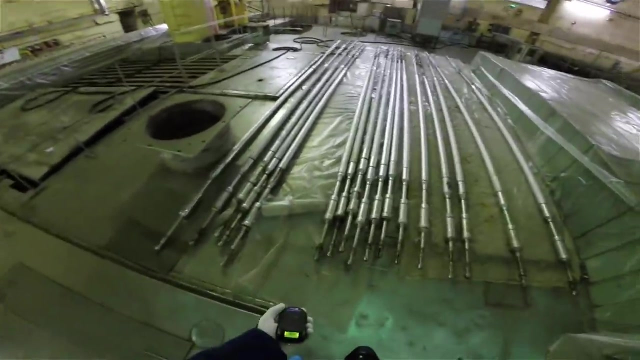 What you see there we'll take another look at later. Those are what I call stringers. They're the holders for things that are inserted into the technological channels. It's all back there, And there are some other ones. These are presumably not used. 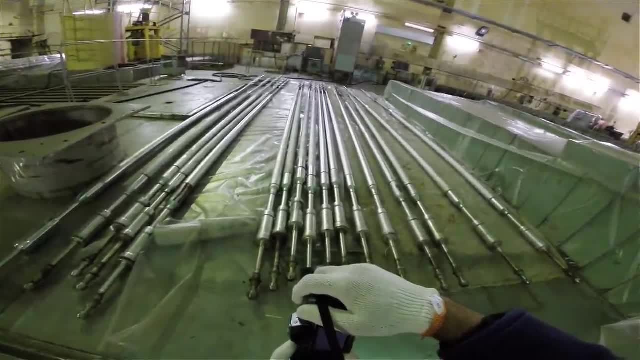 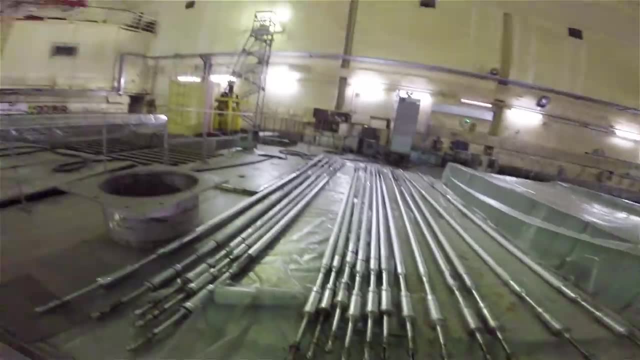 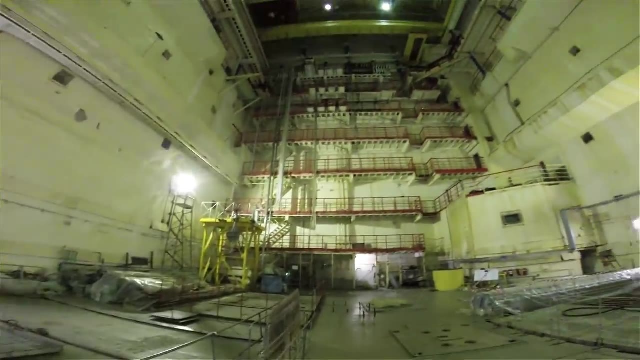 They're not being held in the spent fuel pools, But you can see the little fixture by which the refueling machine grabs the stringer and pulls it out, And ordinarily there would be fuel on the other ends. There's two 3.5-meter long bundles end-to-end. 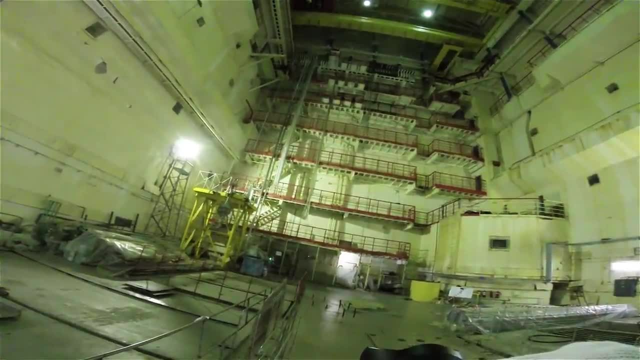 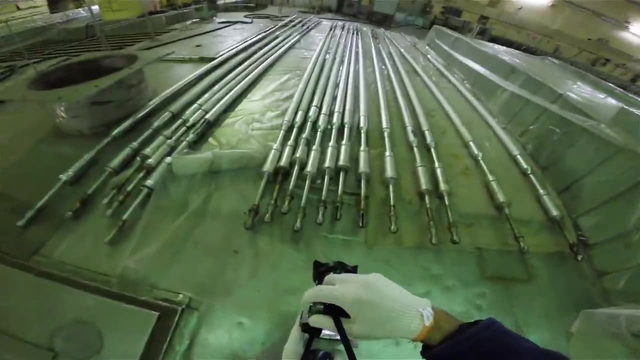 And here's where fresh fuel is stored in preparation for use. Also down at this end of the reactor, down at this end of the reactor hall, is the transfer corridor for fuel. It's just to our left here, And this is where new fuel is brought up. 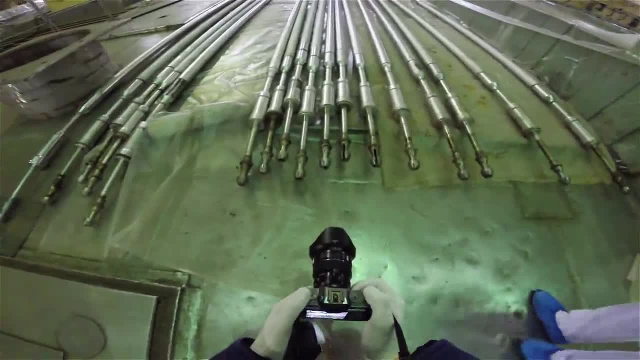 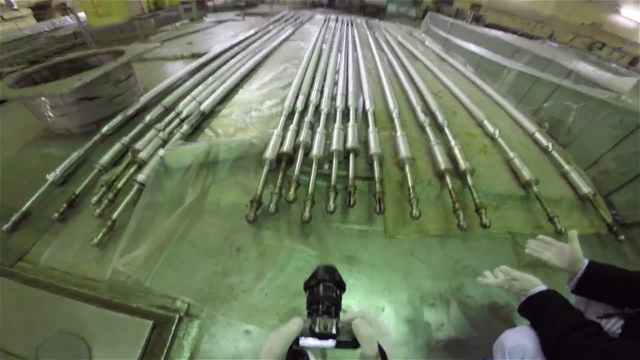 from below. when it's shipped in And also used, fuel can be taken out in a cask. A good view here of the stringer assemblies. This is the top end of the stringer where the machine would grab it. We'll go take a look at some other stuff. 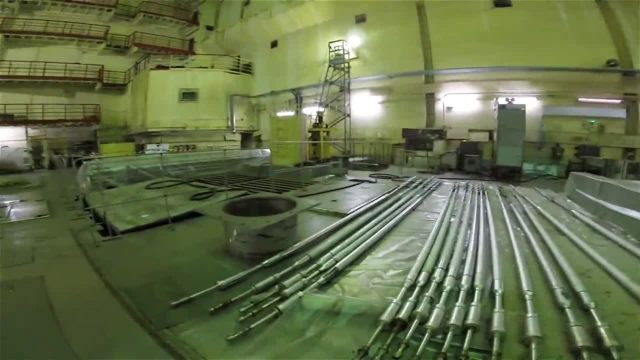 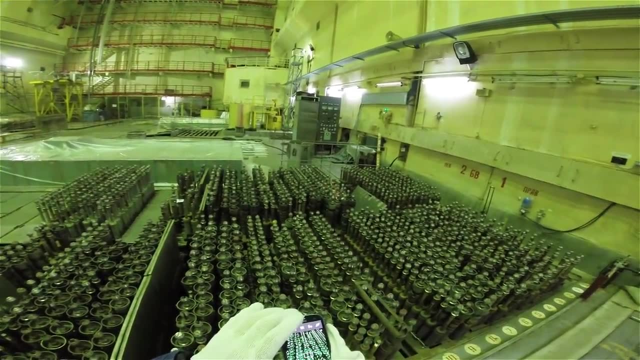 here in the central hall, So I'll go ahead and cut the clip here. This is the spent fuel storage area in the number two reactor And I want to be clear. there is no fuel remaining here. In fact, there's no water in the pool at all. 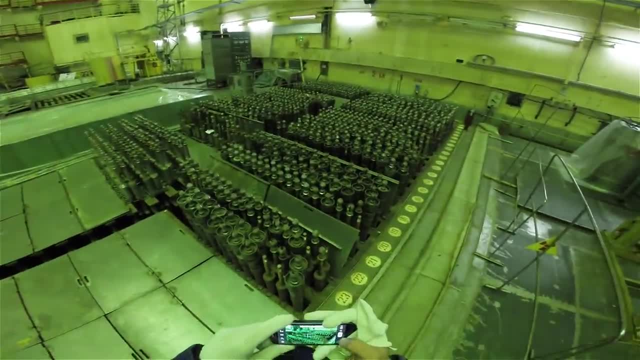 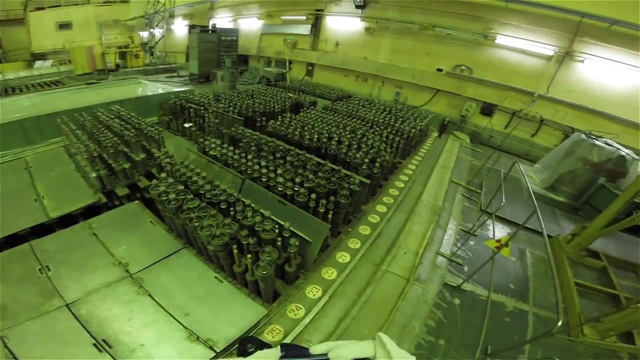 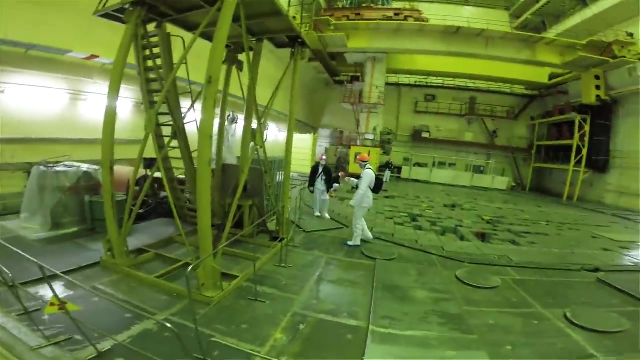 What we have in the pool now are the upper assemblies, the stringer assemblies that would hold fuel in the technological channel if you had the fuel in there. But these stringers are obviously, as I said, not loaded with fuel, But they are radioactive. 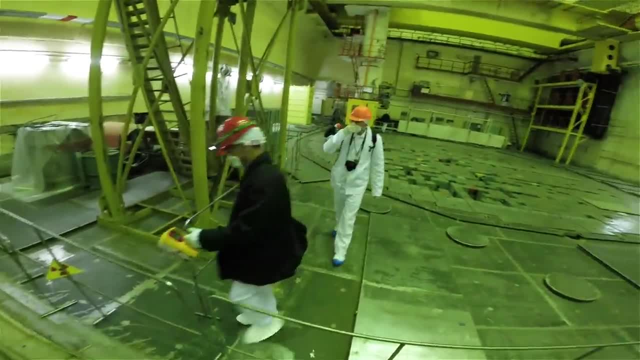 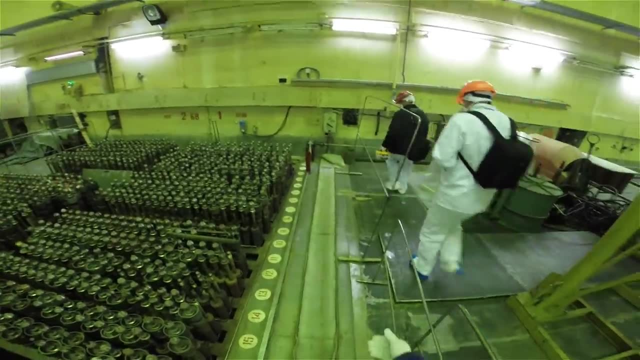 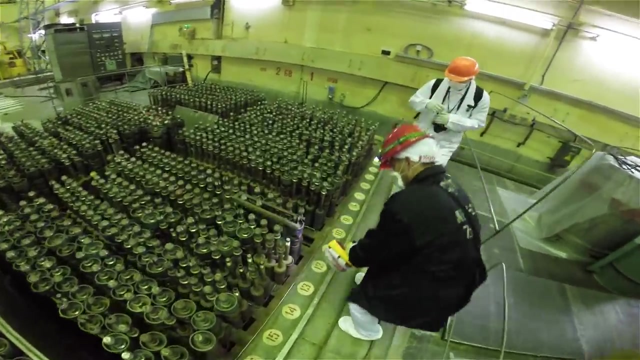 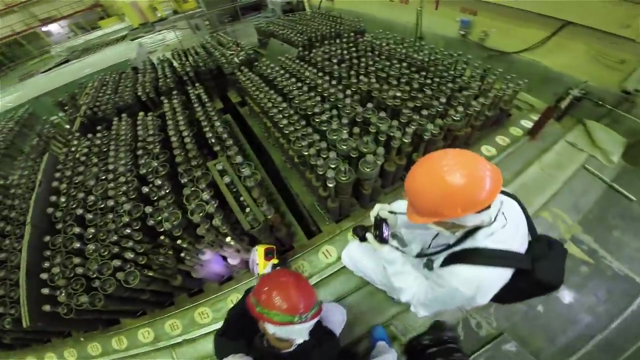 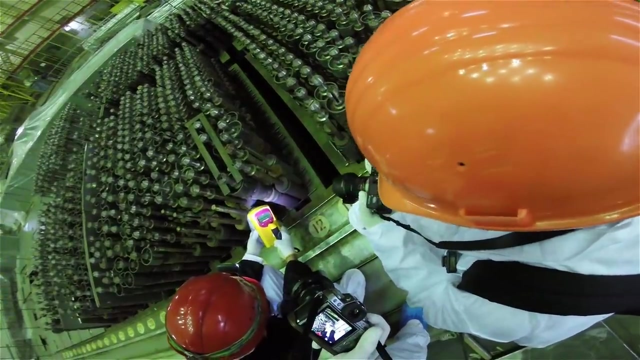 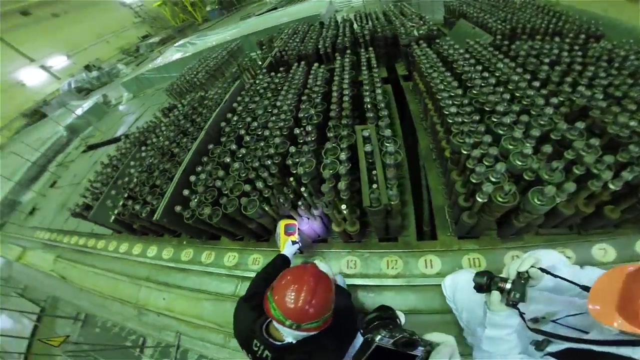 which stands to reason because they're so close to the operating parts of the reactor, And so Lucas has called me over with the ion chamber to look at a hot spot he found here, And we're going to see just how hot it is, And that's the one right there. 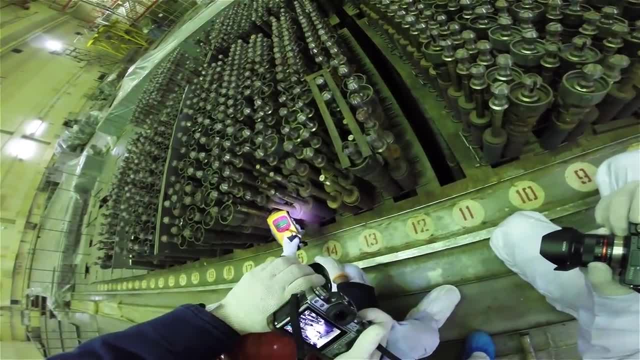 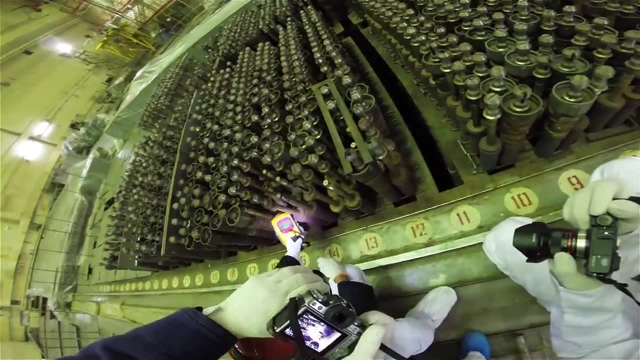 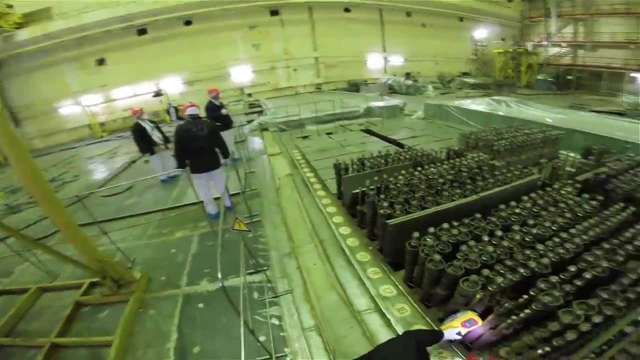 You'll notice, all of these stringers have a nose on them. a little catch that the refueling machine can grab onto in order to drag it out of the channel. It's really- it's quite a clever way of doing things- Incredible. 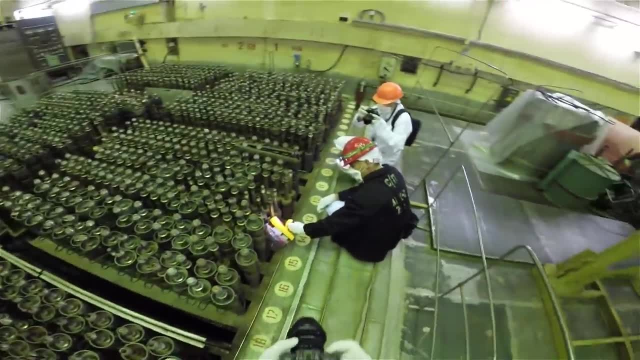 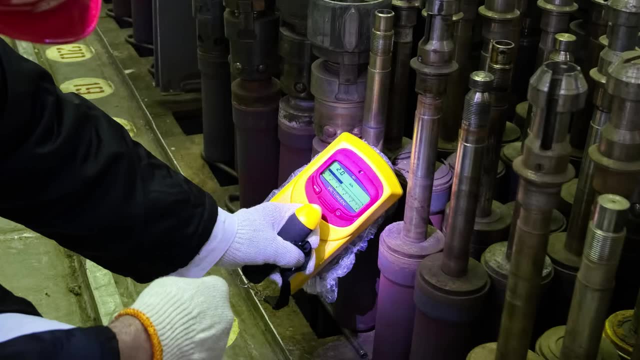 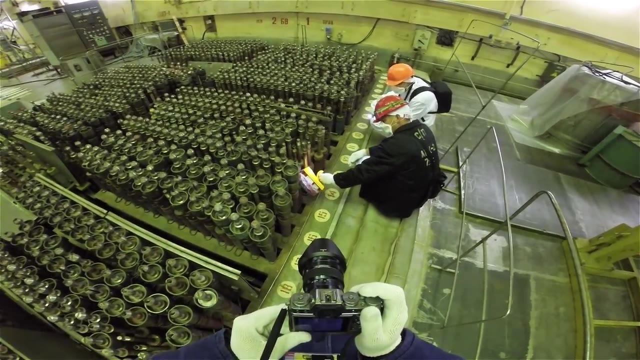 And this spot right here that we're measuring. we're measuring two rentgens per hour And you know this is a power plant that's known for having a lot of spicy stuff around, So two rentgens is really not that high. 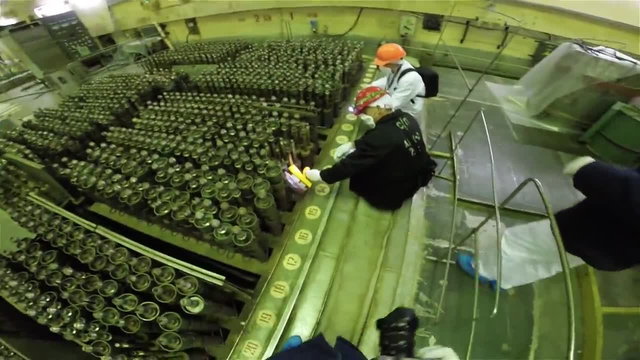 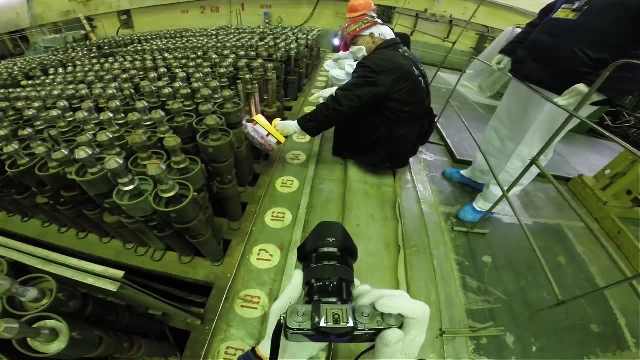 But it's something, And this is, I should be clear. this is very localized. This is not coming from the bulk of all of these stringers that are parked here. It is some sort of fuel flea or just a local bit of leakage. 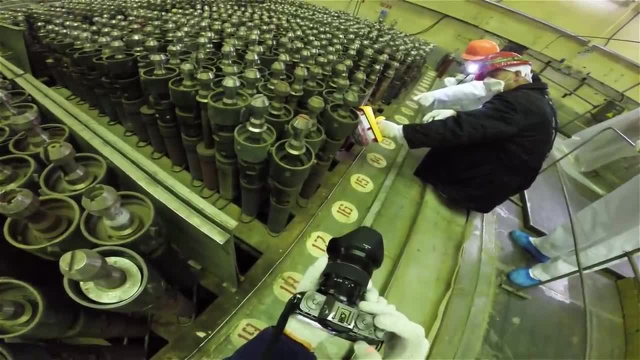 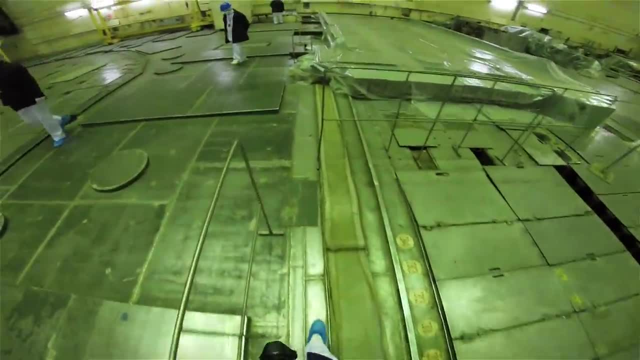 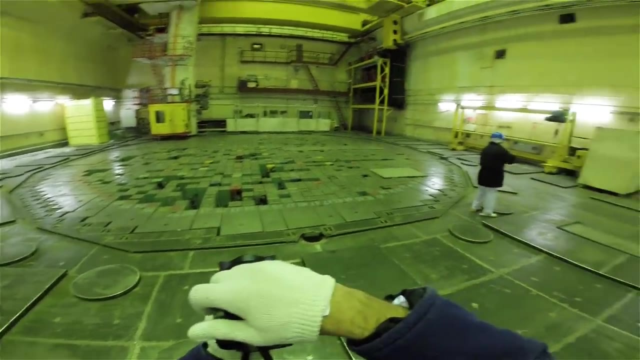 or contamination on that one spot, And so, yes, the dose rate's a little bit high, but it's- at least as far as this power plant is concerned, it's really not Not much at all. Stanislav, how many times have you been in? 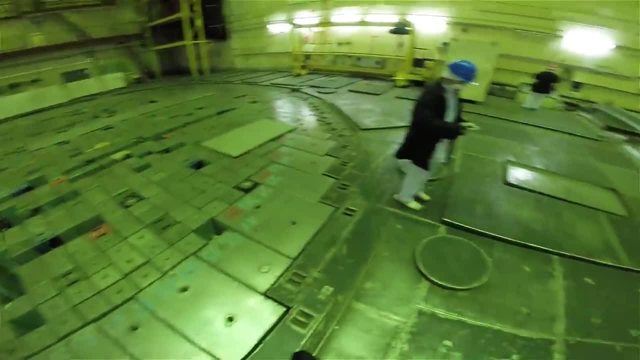 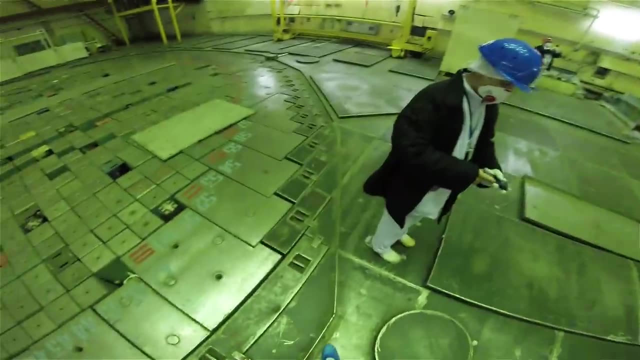 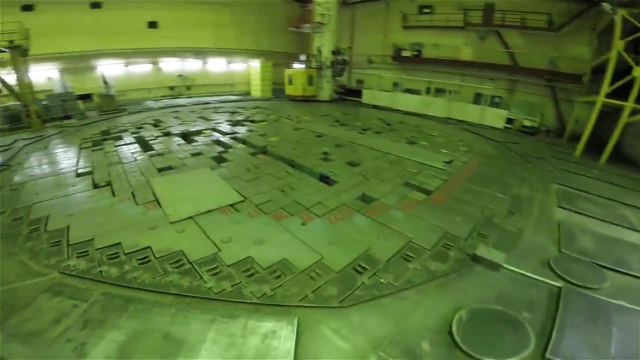 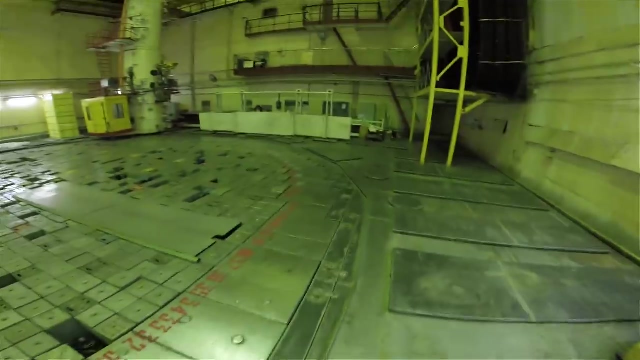 in here Many? Yeah, Is it okay if I walk up on the scaffolding now that everyone is down? Yeah, Thank you. Thank you, This is incredible. Oh, this one right here. Yes, So now we're going to go up. 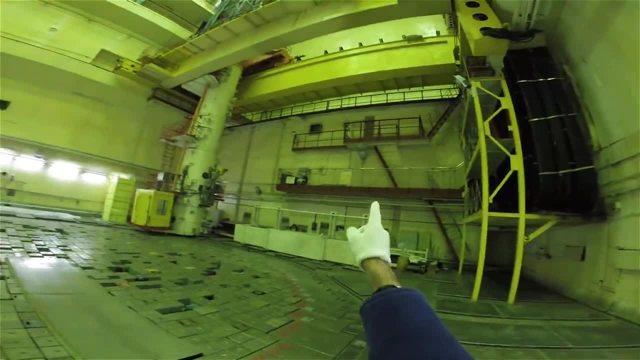 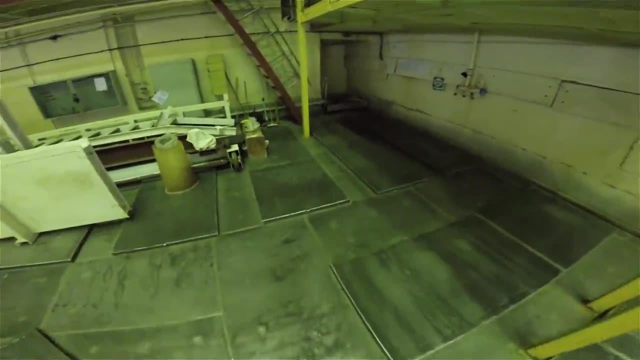 and look at the refueling machine operator's room And, as mentioned before, the central hall of these reactors is basically a large hot cell because when spent fuel comes out of the core into the refueling machine, there's a lot of radiation in there. 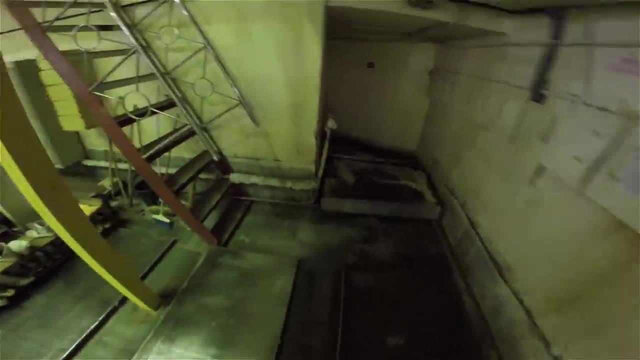 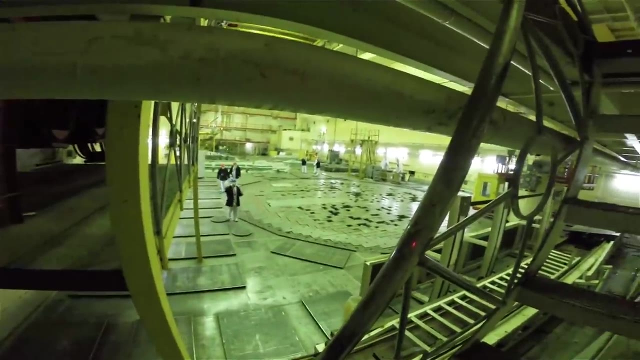 So you know there's a lot of radiation in there And you know there's a lot of radiation in there, And you know there's a lot of radiation in there And you know there's a lot of radiation. 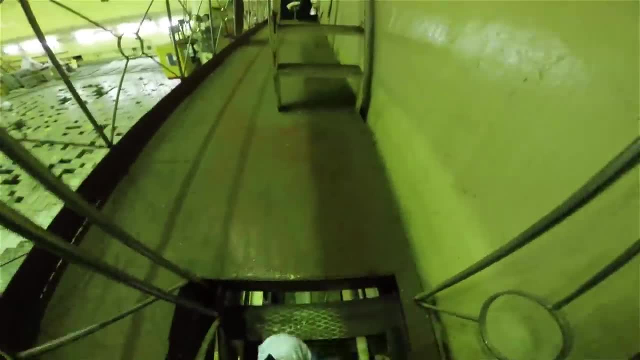 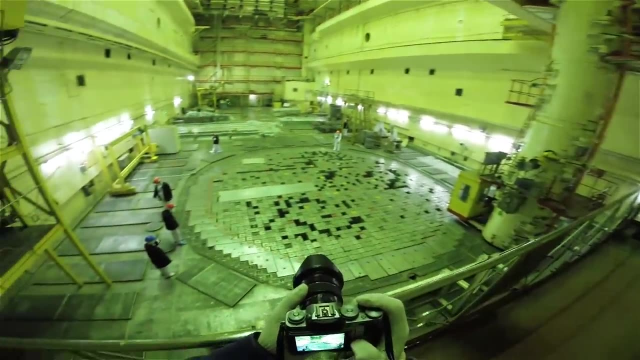 in here, And so the operator sits in a little booth behind a leaded glass window, and we'll go take a look at that shortly. But right here, while we're up and have a up on the balcony and have a good look down at the core, 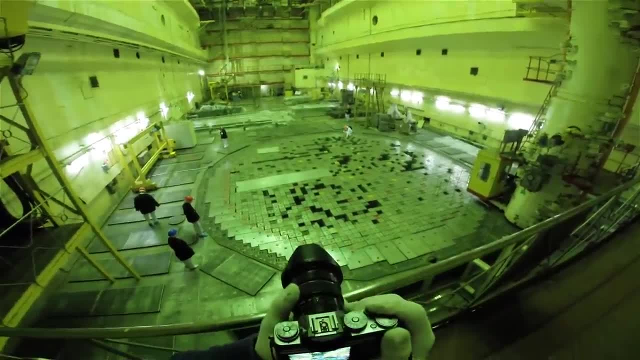 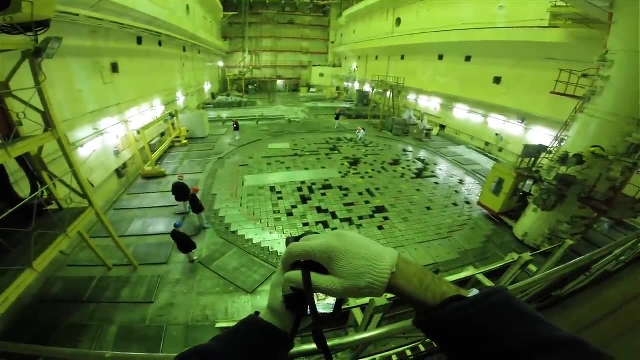 I'll just mention a few things. There are about 2,000 penetrations vertically through the RBMK core, And some 17 of the 100 of them carry nuclear fuel. These are the so-called technological channels. And and then we have 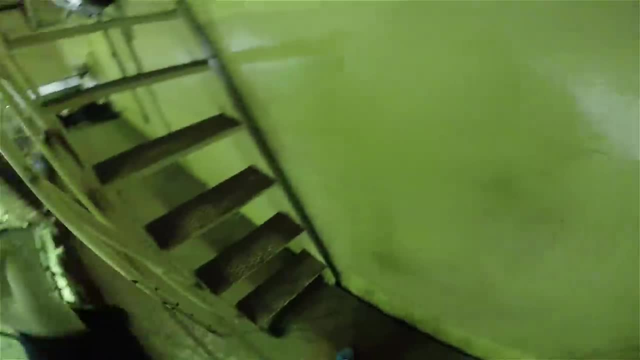 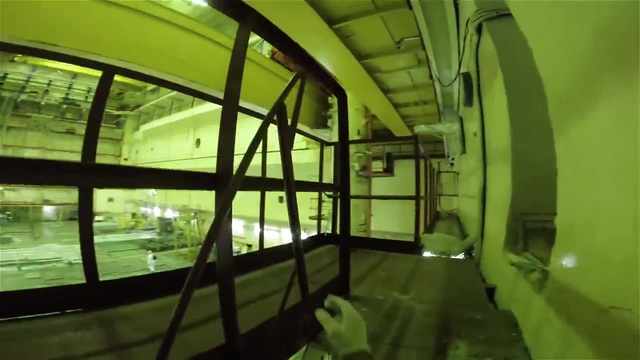 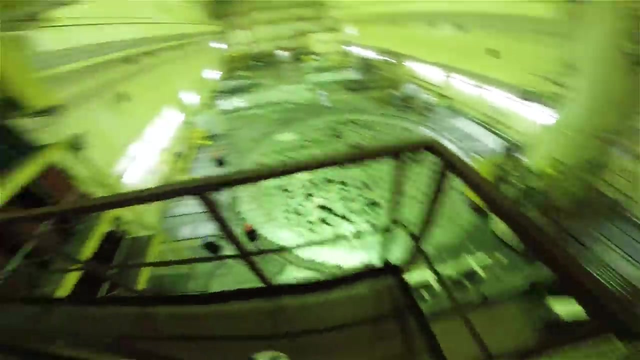 200 more that contain control rods of various types. The control and protection system has rods that descend from the top of the core. It has short absorber rods that come from the bottom of the core. There are rapid shutdown rods, the BAZ. 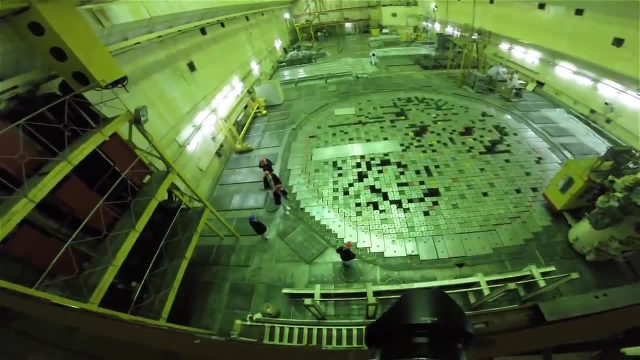 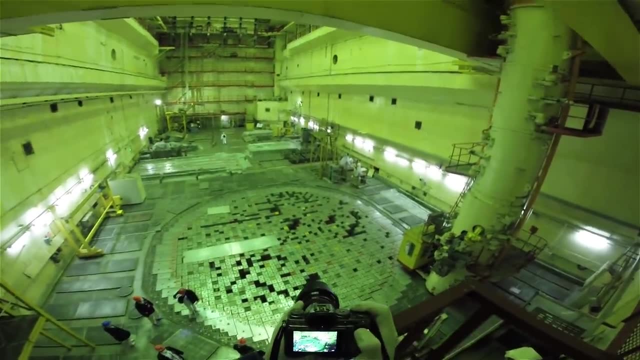 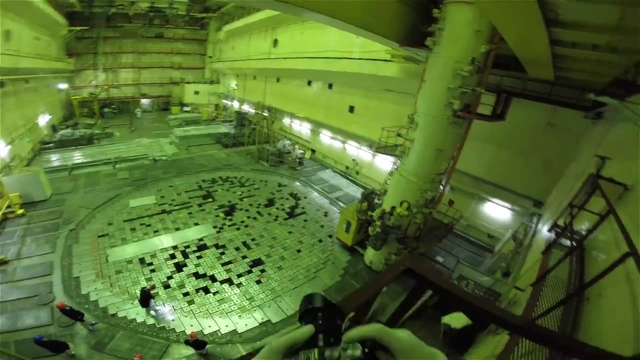 system rods that come from the top, And there are. there are regulating rods as well as emergency shutdown rods that are used to control the control systems. It's really quite a complicated arrangement And in this reactor at least, and in the number three unit, 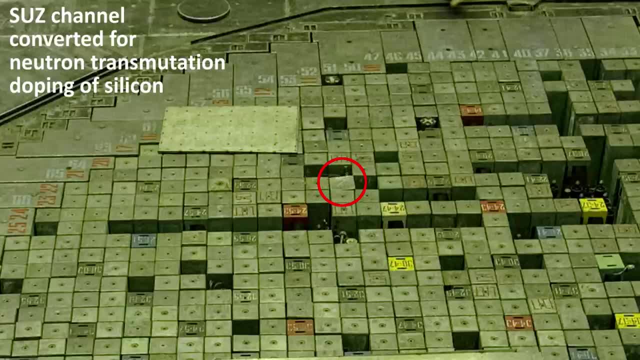 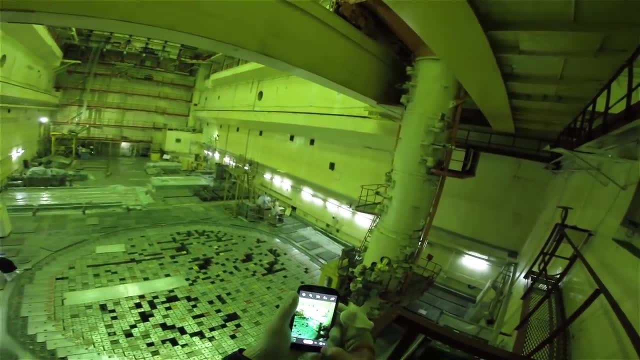 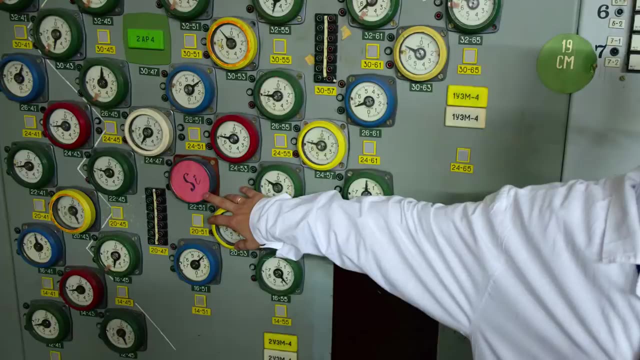 at here at Chernobyl. one channel that belongs to the control and protection system has actually been set aside for radia for neutron doping. activation doping of the servo indicator indicated that it was being used for silicon rather than a normal control and protection. 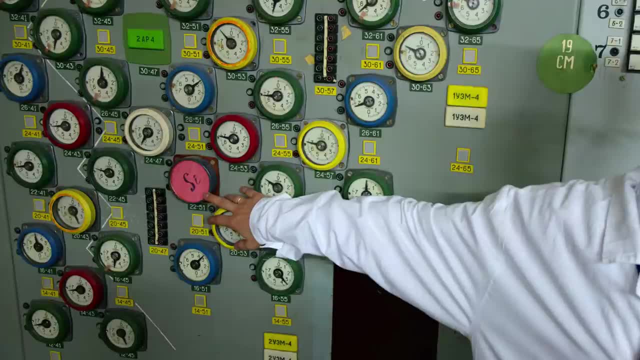 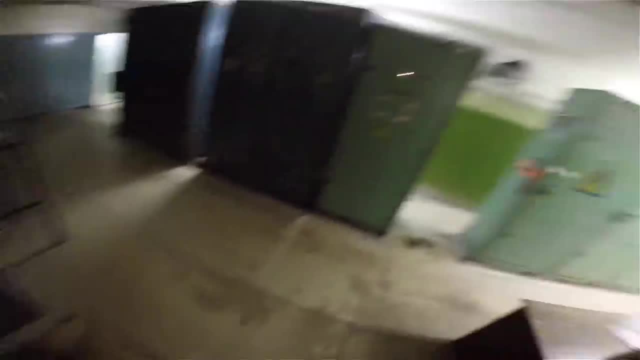 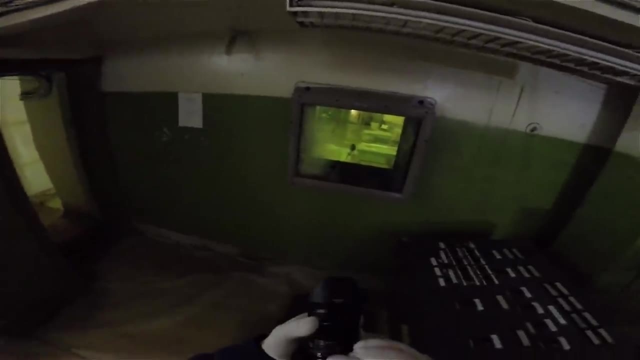 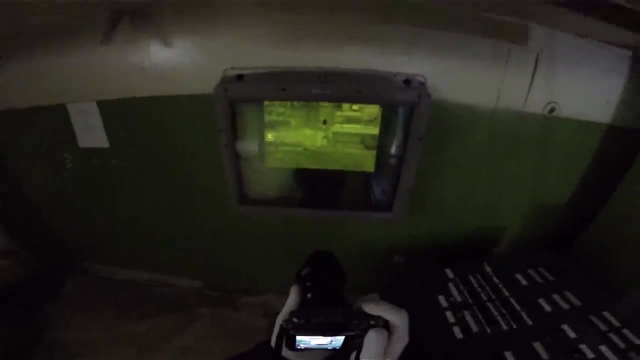 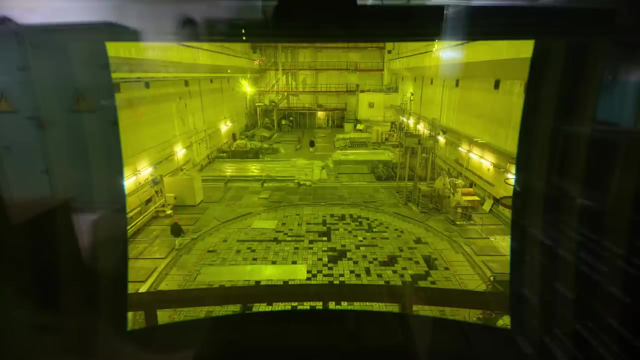 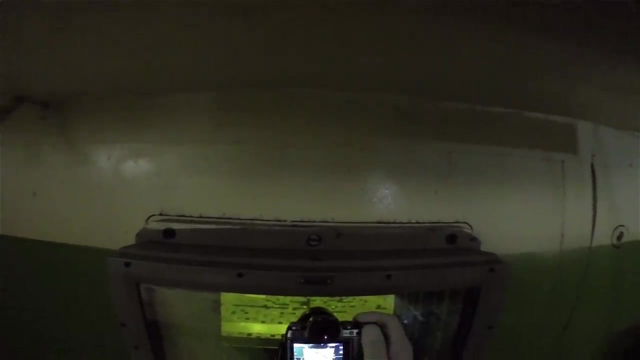 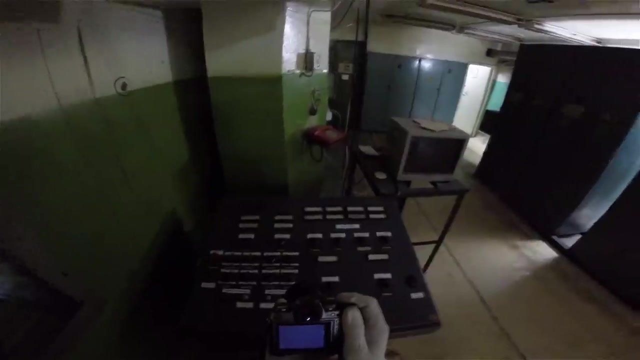 system channel, And here in the photo you can see exactly which one that is. Now we're going to go into the booth here where the refueling machine operator sits, and you can see the window that operator looks through when he's working. So, Lucas, 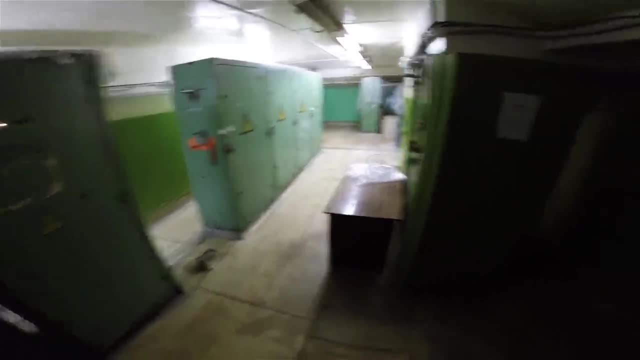 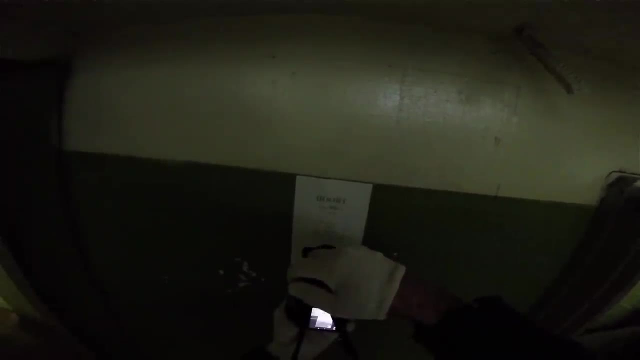 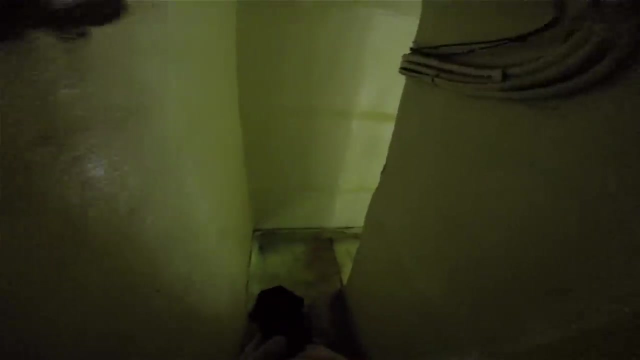 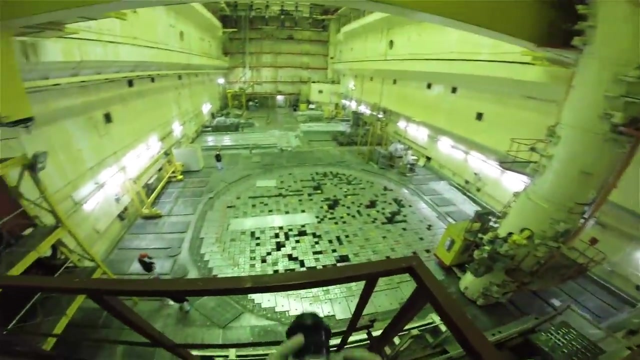 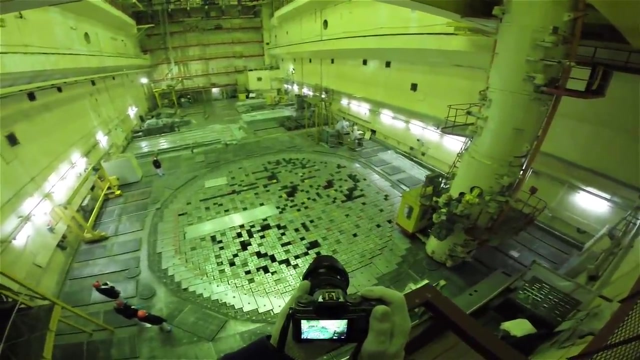 is getting photographs of literally everything in here and now we'll head back out through the shielding maze, back out onto the platform here, And this is a good view of the reactor and this is a good view of the central hall In the distance behind the. 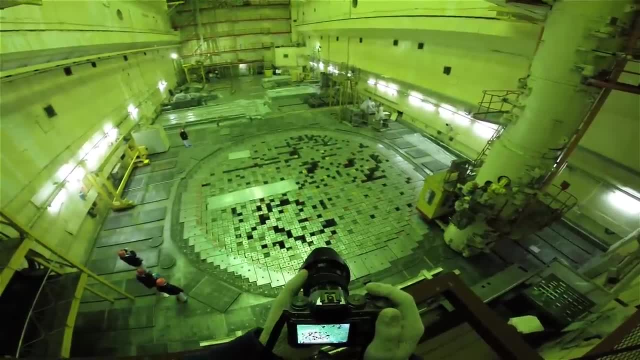 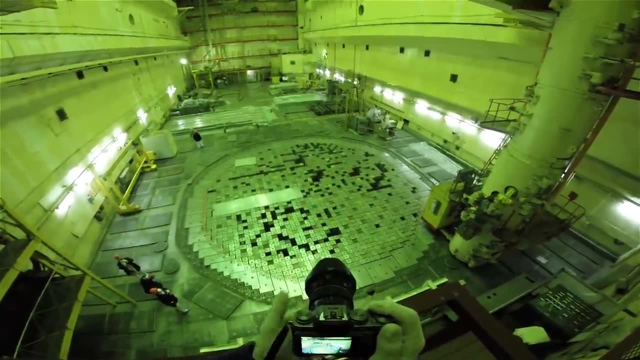 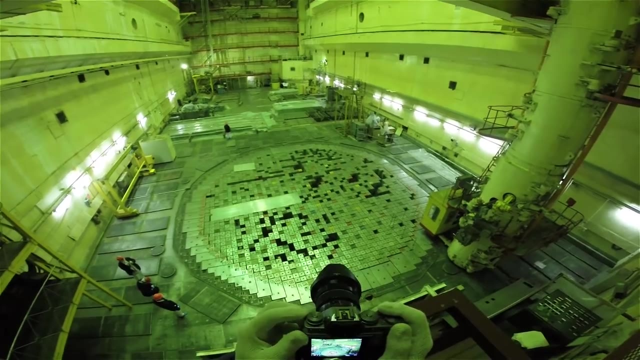 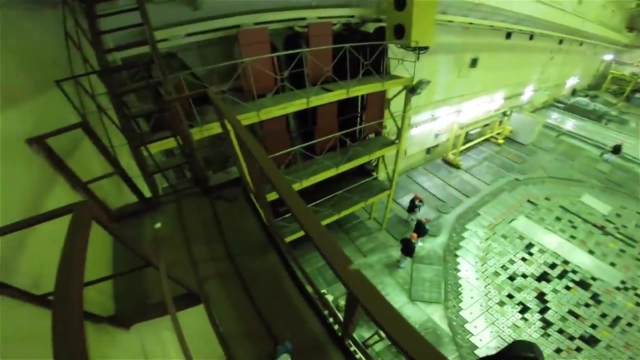 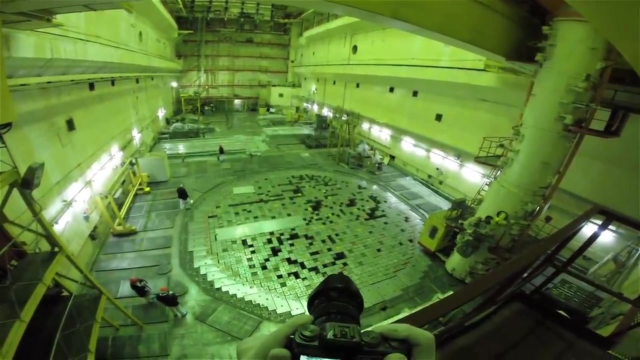 reactor. we have the two spent fuel pools on the left and on the right and then behind them along the central axis of the room. here is the fuel transfer corridor, which is a round of the reactor, and this is a very good view of the reactor fueling. 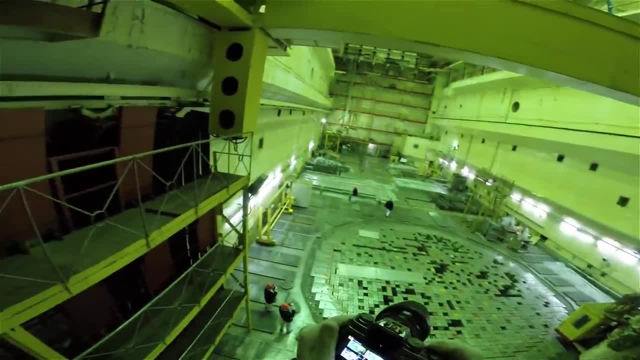 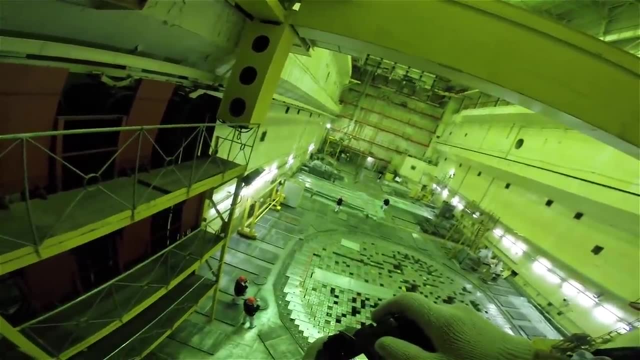 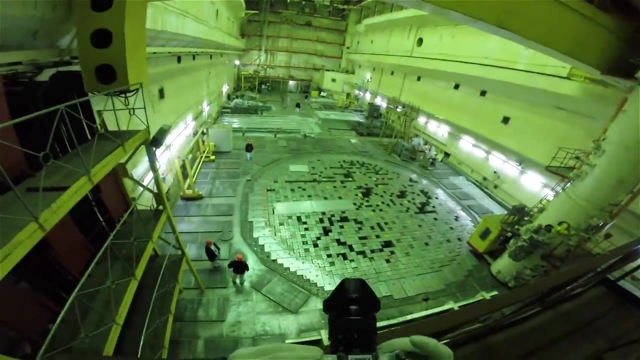 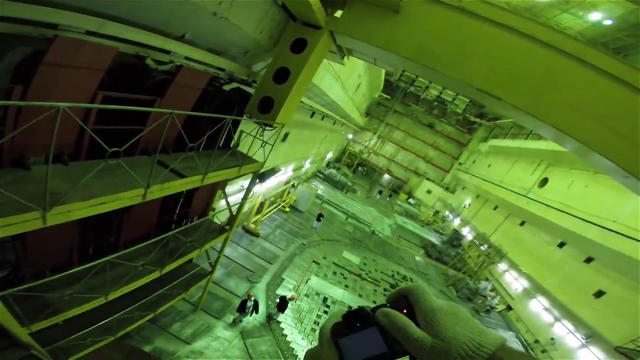 phase in Chernobyl, Unit 2.. This reactor has been offline since the accident in 1991. that basically, And it was a political decision not to restart the No 2 reactor but to leave it shut down, And it's been that way ever since. So the history of this place, even though the lights are on and it's quite pretty in here,